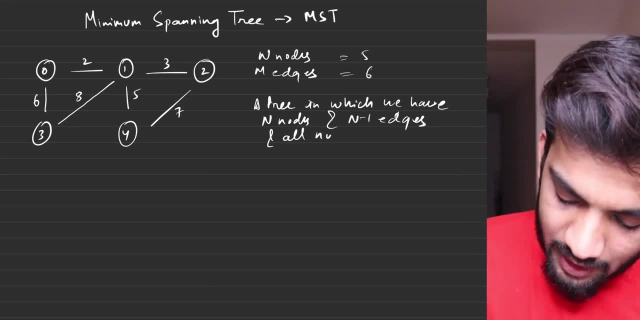 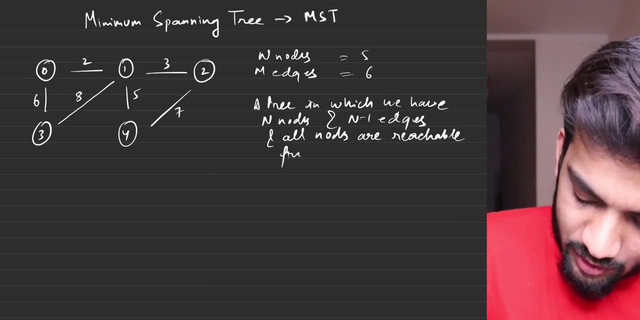 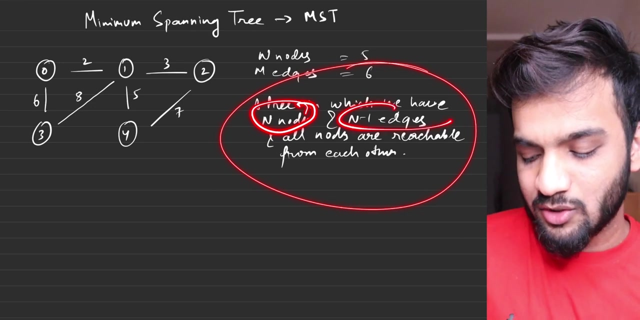 or N minus 1 edges, and all nodes are reachable from each other, and all nodes are reachable from each other. So if someone does ask you the definition of spanning tree, please make sure you tell them that it should have N nodes, N minus 1 edges, and all nodes should be reachable from each other. That is the definition. 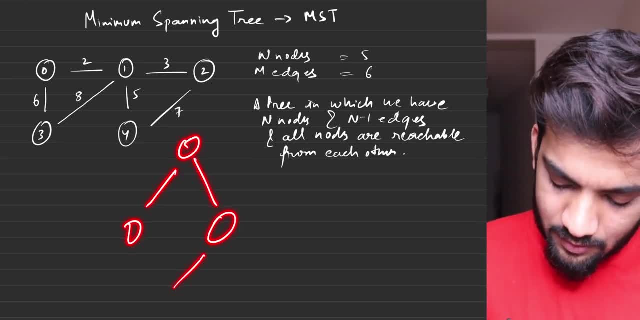 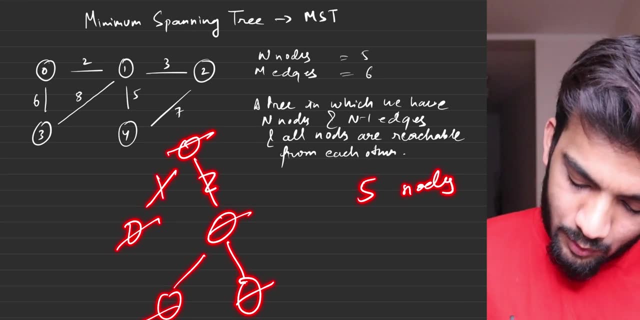 of a tree. So if you remember a tree, like if I draw a tree, so what is this tree? 1,, 2,, 3,, 4,, 5,, 5 nodes. And if you carefully see 1,, 2,, 3,. 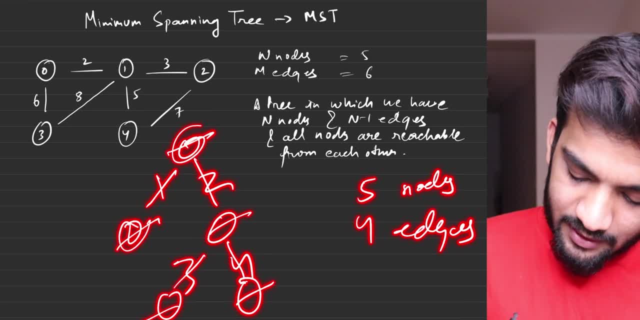 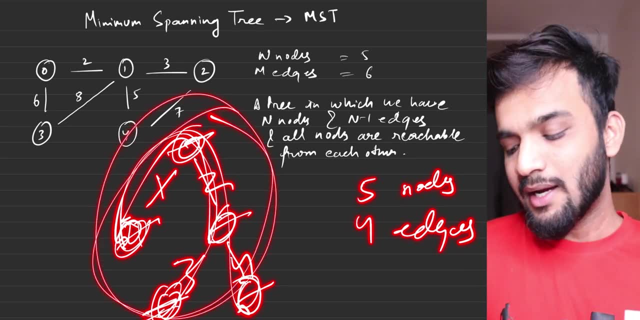 4 edges and everyone is connected to each other. If you want to go from here, you can go. If you want to go from here, you can go. If you want to go from here, you can go. So everyone is connected and it has exactly 5 nodes and one lesser number of edges, So that 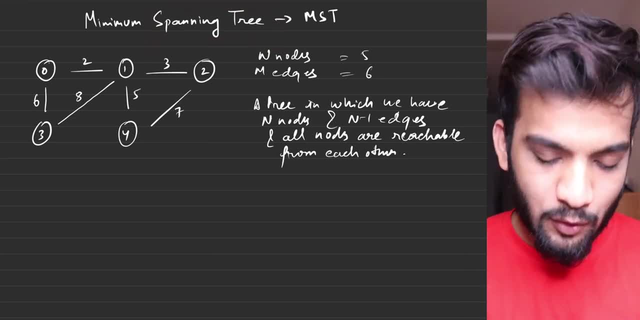 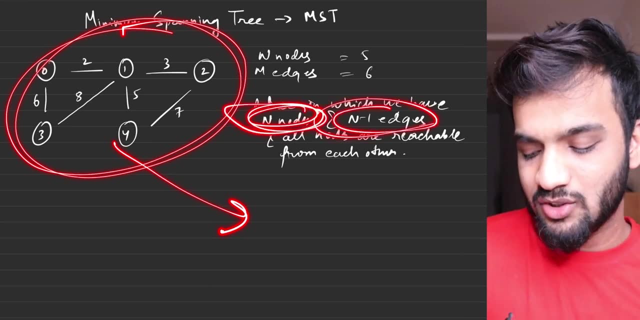 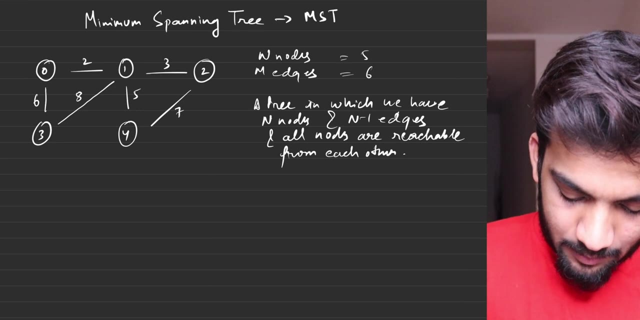 is what the definition of a spanning tree is. You have to make sure that from this you draw a tree out such that it has all the N nodes, N minus 1 edges, and all nodes are reachable from each other. example: if I try to draw one of the spanning trees, it can be something like: I will take zero. 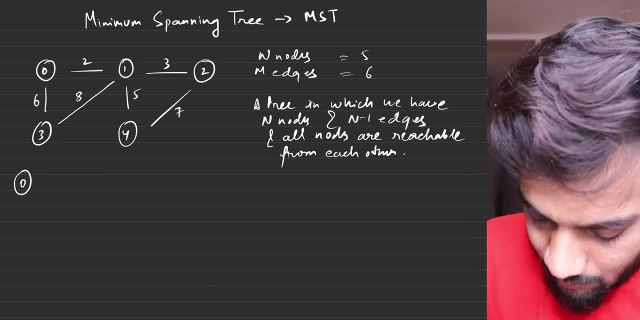 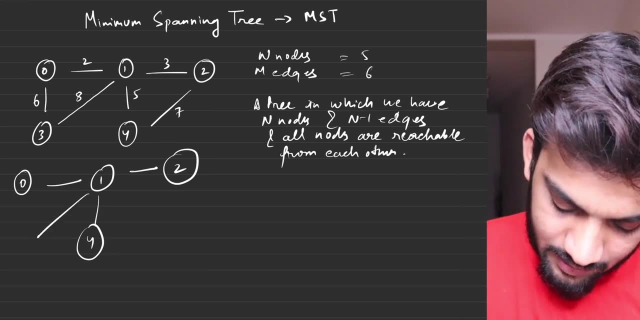 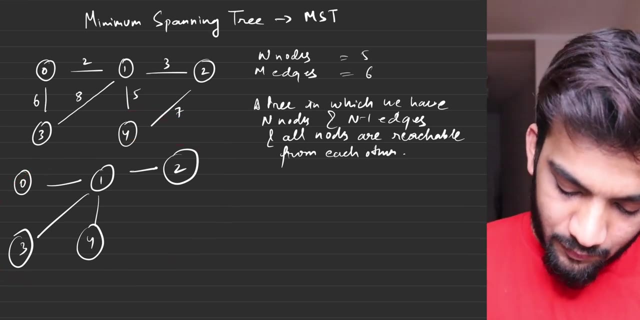 I will probably take one with it, and I'll take four, and then I'll take two, and then I can definitely take something as three. so can I say this is a spanning tree? I definitely can say that this is a spanning tree. why? because if you look one, two, three, four, five, five nodes, and if you 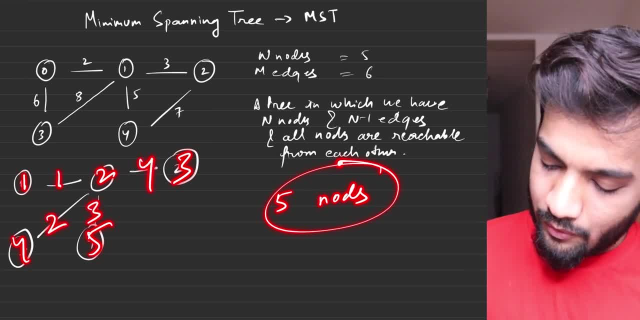 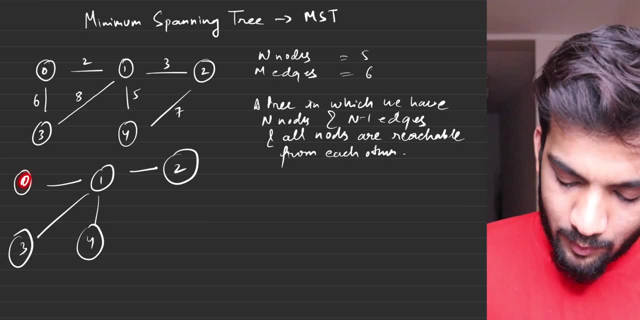 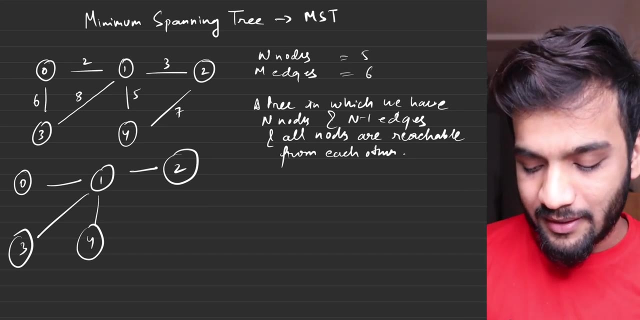 carefully see the number of edges- one, two, three, four, four edges- so thereby this can be called as a spanning tree. and if you carefully observe everyone, all the nodes are connected. everyone is in a component, is in a single component. thereby this can be called as a spanning tree. 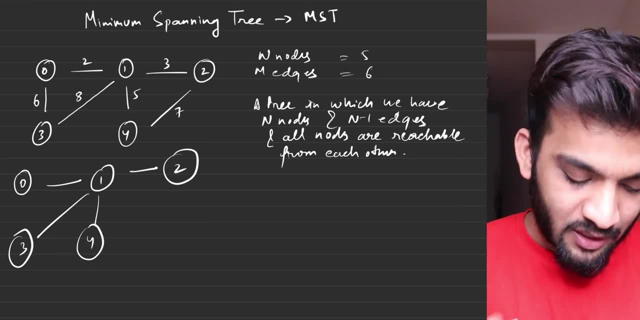 can I draw a few more spanning trees from this particular graph? yes, we can assume I take three, assume I have something like a one, assume I have something like a zero and I can draw one second, one second acting as a spanning tree. and if I draw two, 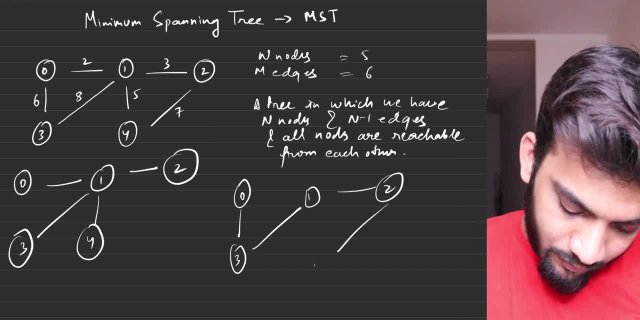 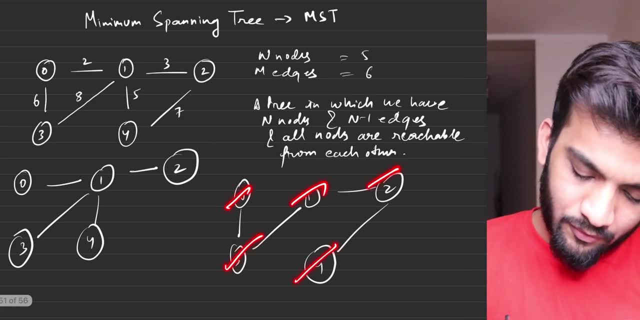 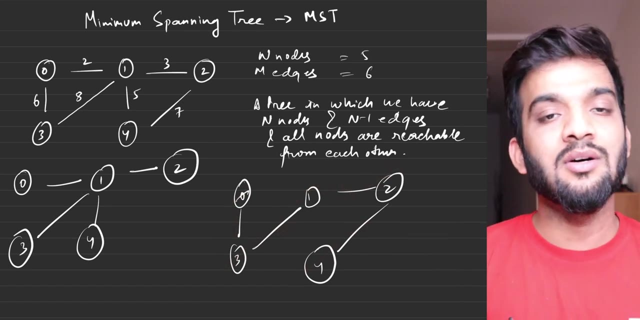 zero, and then i have something like a two and then i have something like a four. this is also spanning tree. why? because if you see, we have one, rather we have one, two, three, four, five and one, two, three, four edges, five nodes and four edges again. similarly, can i draw any other spanning tree? yes, 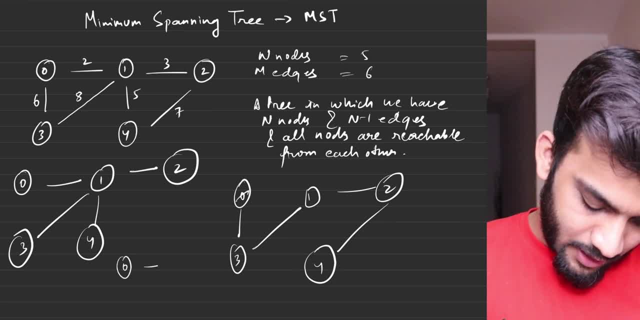 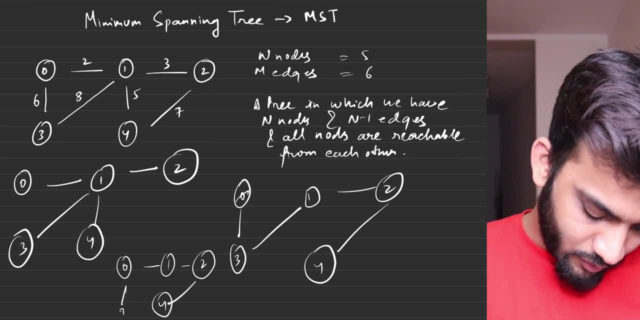 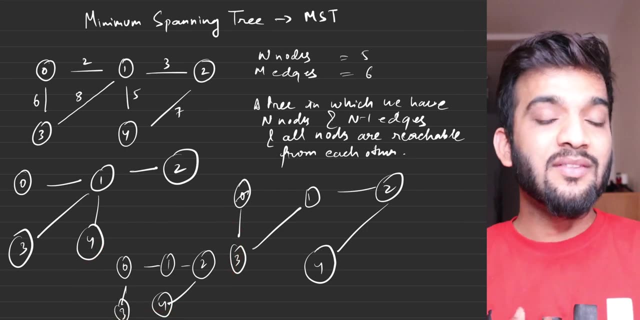 i can draw how. imagine i take zero and then i take one, and then i take two and what i can do is i can probably relate four over here and i can have three over here. this is also a spanning tree. why? because, again, one, two, three, four edges and all the nodes are connected. so in this way you can have 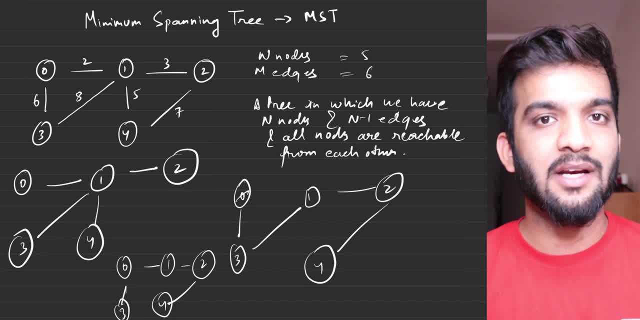 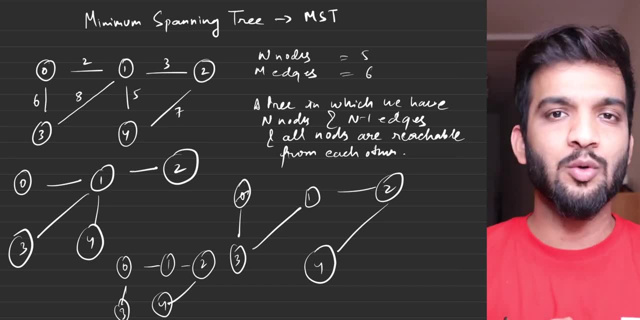 a multiple like. there is no restriction on the number of spanning trees. you can have any number of spanning trees depends on graphs. any graph might have one spanning tree, some graph might have two, some graph might have three, some graph might have five. there is no restrictions, it depends. 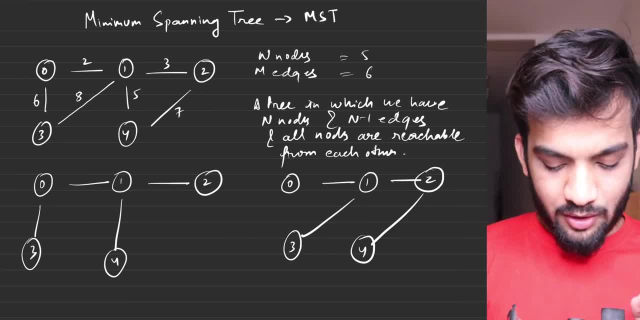 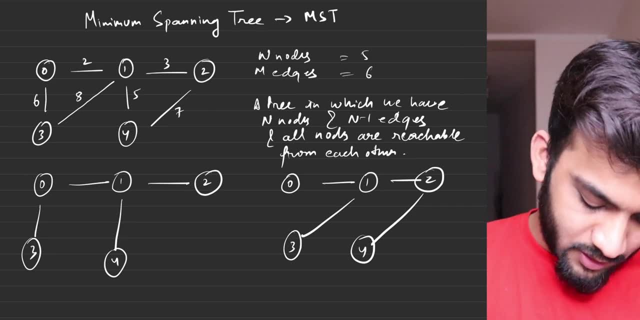 on a graph to a graph. so i've drawn on two spanning trees. one is this one, while the other one is this one. now what you need to do is you need to write the edge weights. so imagine, i write the edge weights: it is 6, this is 2, this is. 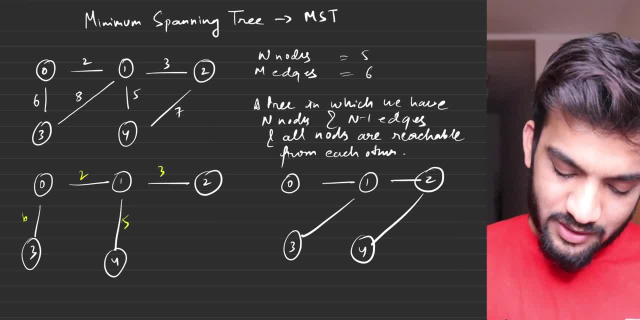 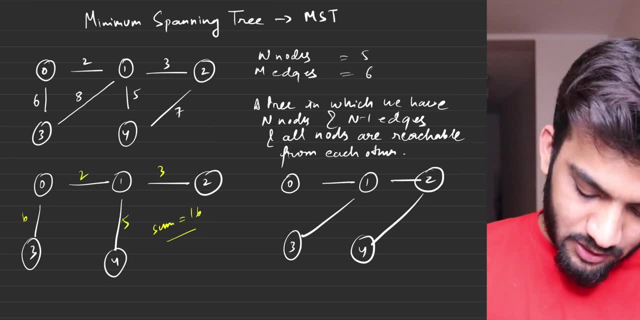 5 and this is 3. okay, if i sum it up, 6 plus 2 is 8 plus 3 is 11. so the sum of all the edge weights is 16 in this case. okay, if i write the edge weights over here, it's 2, it's 8, it's 3, it's 7. 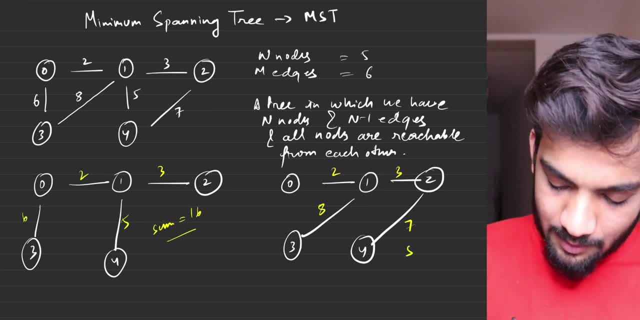 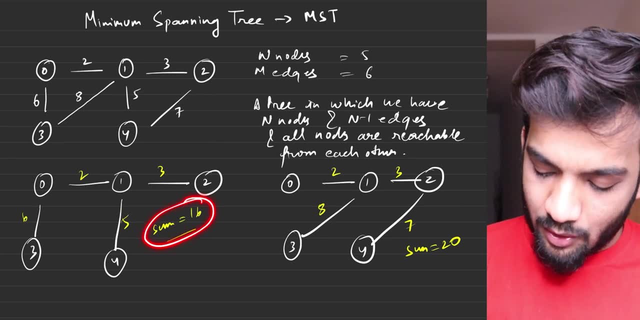 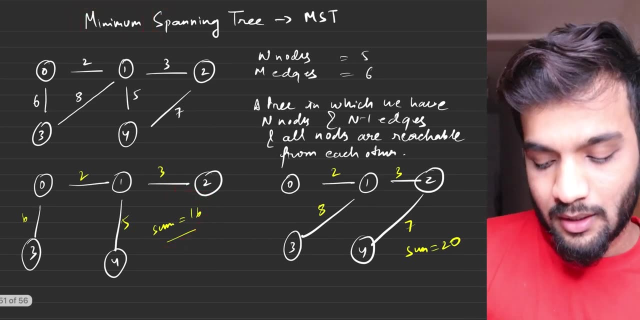 and if i try to sum it up, it's basically 10, 3, 13 and the sum comes out to be 20. so you can draw all the spanning trees, you can draw all the spanning trees and you can figure out the sum. okay, now, the tree which has the least or the minimum sum will be the mst of this particular 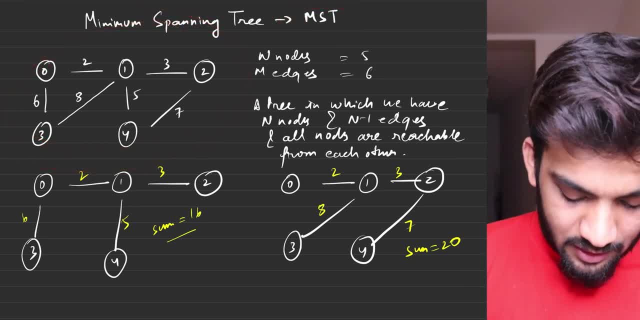 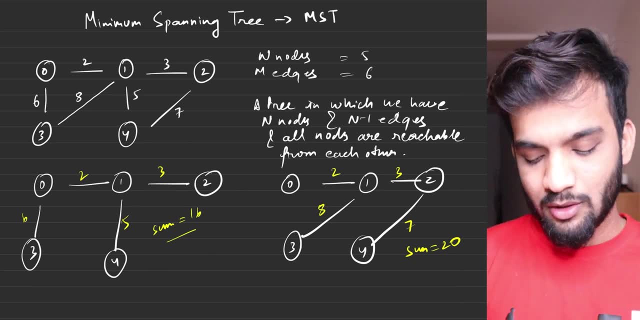 graph. so, for this particular graph, what i can say is: this is the mst why? because the sum is 16. you can try drawing out all the other spanning trees. you can try drawing out all the other spanning trees. you can try drawing out all the trees, you'll find that this is the spanning tree which has the least sum Can a graph. 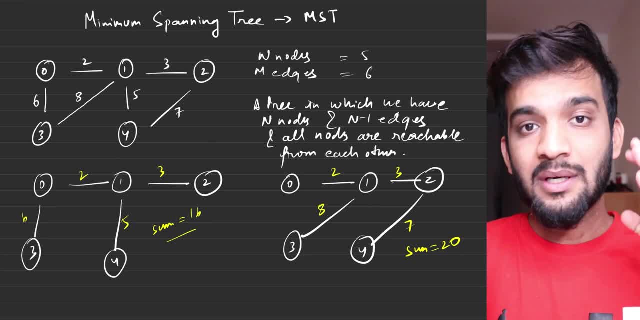 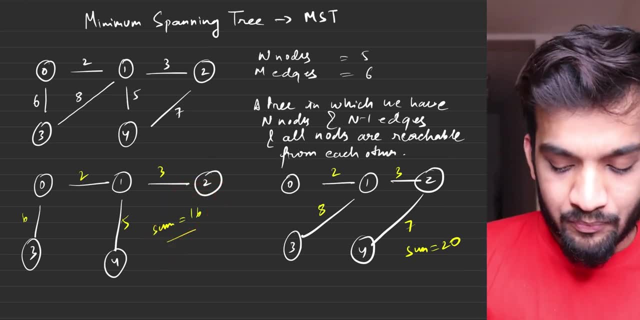 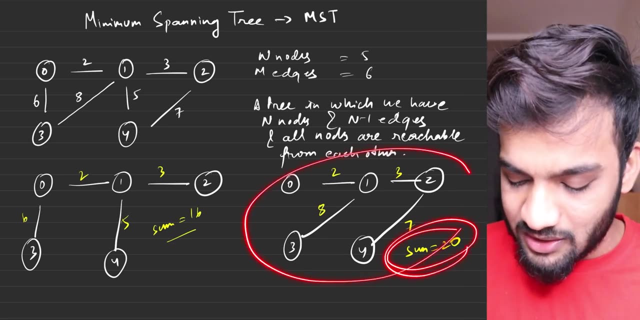 have more than one spanning trees? Yes, it can have, but the idea is any tree, any tree with the least sum, any tree with the least sum is called the MST. It can be two, it can be three, but the sum has to be the least. You cannot say 20.. You can call this as a 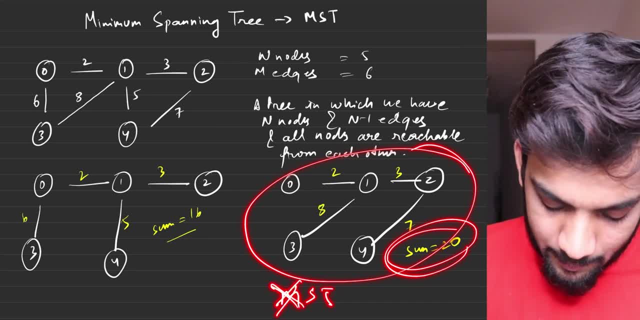 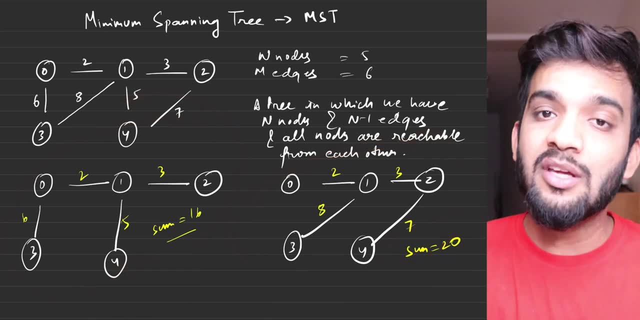 spanning tree, but you cannot call this as a minimum spanning tree. but you can call this as a minimum spanning tree. You need to understand this is a spanning tree, but this is a minimum spanning tree. Any tree which has the minimum sum is known as MST. 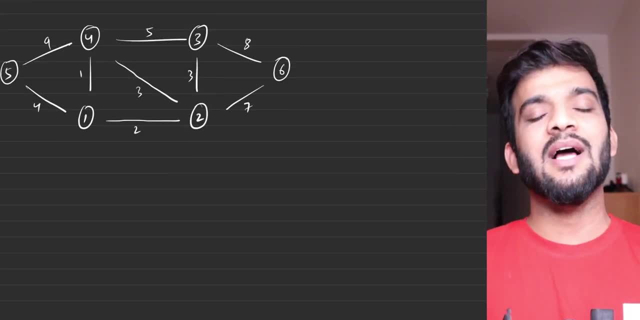 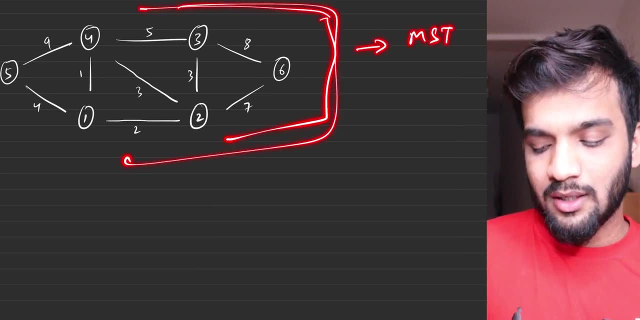 I hope the definition of MST is clear to you. So, in case MST is clear, I'll give you a very, very small task. So this is a graph that I'm giving you. What you need to do is you have to draw the corresponding MST of it. So I'll also be drawing it, but you need to pause. 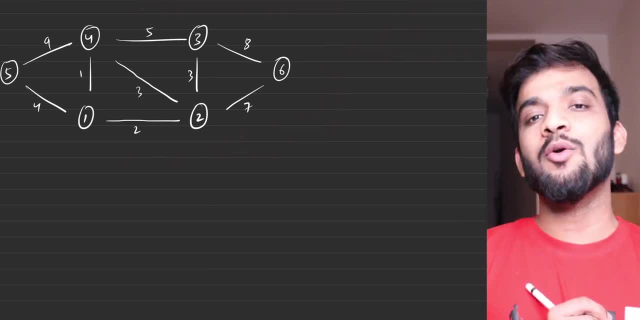 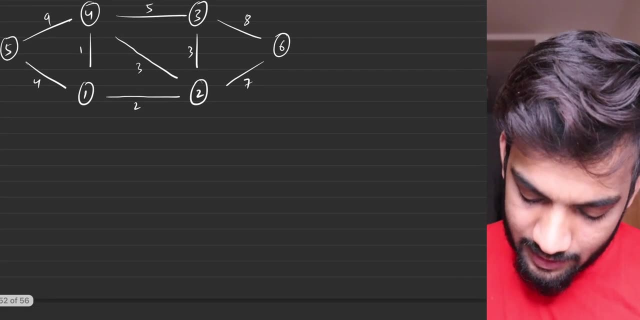 the video. now draw the MST. come back and start drawing. Check out my answer. Okay, So what will be the MST for this particular graph? It's very simple. What I'll do is I'll first take one and probably I'll connect it with four Then. 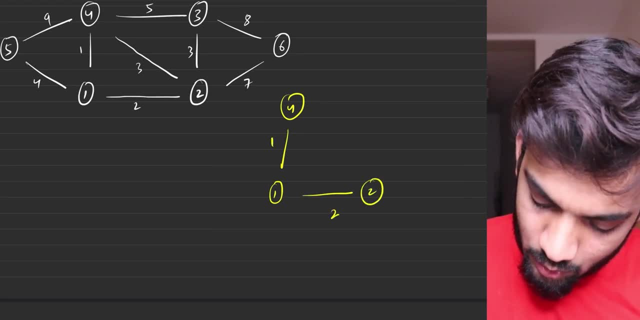 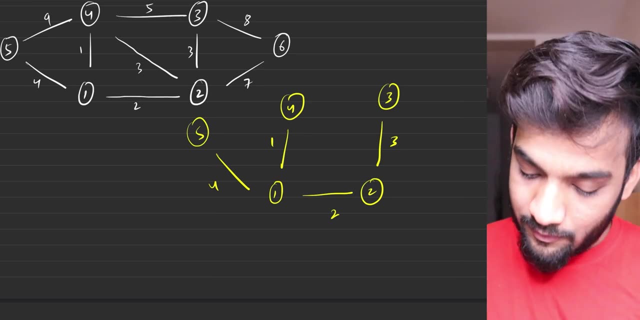 I'll connect it with two, That'll be edge weight one, two. I'll try to connect with three, which will give me an edge weight of three. Then I'll try to connect with five, which will give me an edge weight of four, And then I'll try to connect with six, which 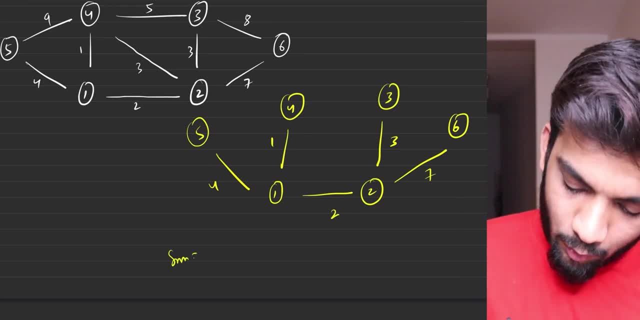 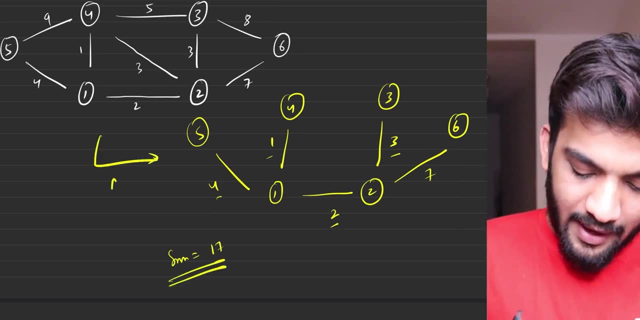 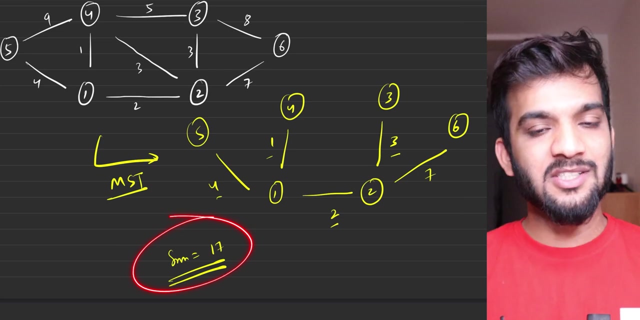 will give me an edge weight of seven. So I think sum will be four plus one. five plus two, seven three, Sum will be 17 for this particular MST. Okay, So you can try it. try out on your own as well. So in case you also got the same MST, perfect, Just in case you. 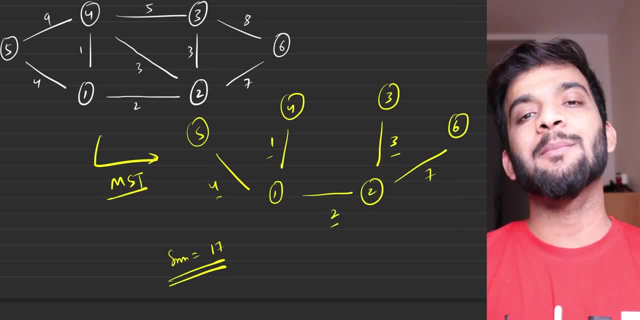 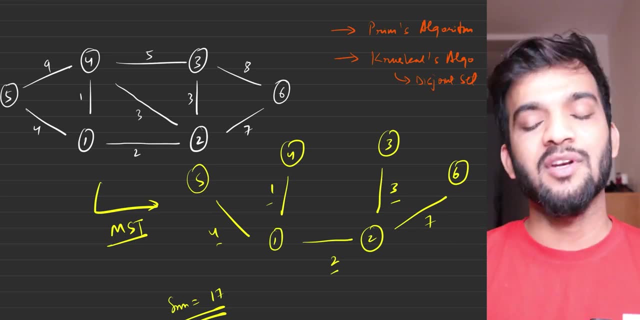 did not nothing to worry With more and more examples in the upcoming videos, MST will definitely get clear to you. So now you must be thinking: how do we find the MST of a given graph? Very simple, There are a couple of algorithms. One is the prims algorithm, which 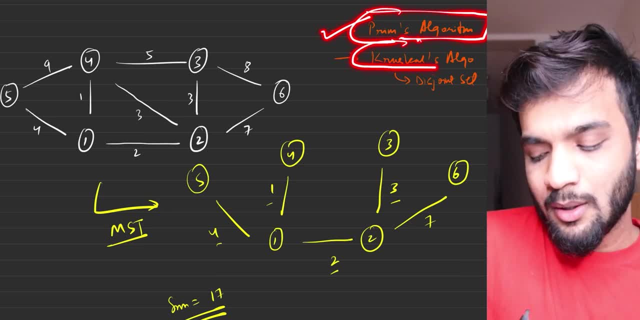 I'll be discussing in the next video. And the other algorithm is the Kruskal. But in order to understand that, you have to know disjoint, set data structure. In the next video let's learn prims And then we'll be diving.